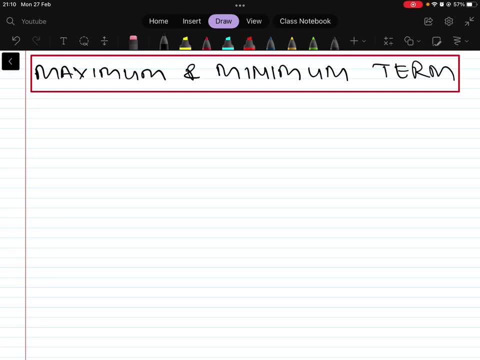 hi, welcome back to the video series. so in this example, or this video rather, we are going to be looking at maximum and minimum term. this is usually a quick question when you are dealing with number patterns. it usually pops up in either question one- I mean question two- or question three of your paper one. 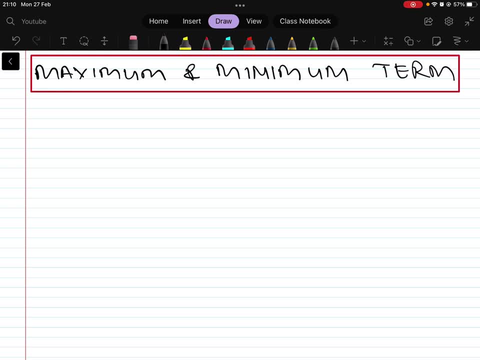 formats. so I'm just gonna look at how many examples. it's about ABC and D. that's just four examples and then we are done. so one thing I need you to understand is that this kind of questions they are only applicable to quadratic sequences or series or number patterns, only applicable to quadratic. 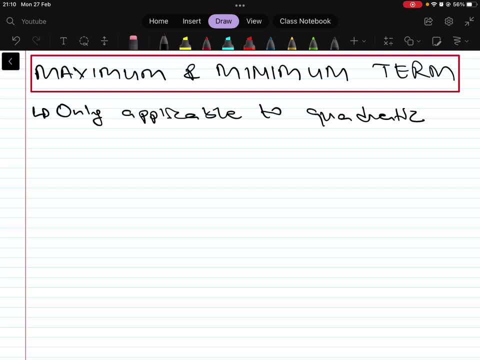 procedures. so with the quadratic, you remember quadratic basically just means parabolic, because if you remember the equation of a parabola, it's y equals to Ax squared plus Bx plus C. so with quadratic, the general equation that we are saying is Tn equals to 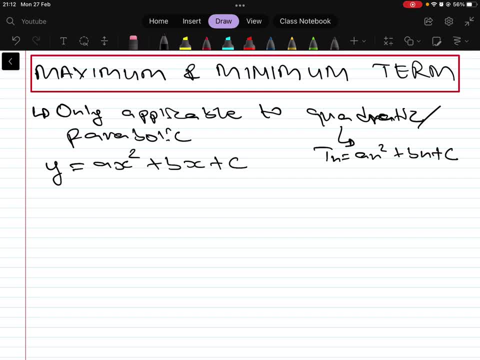 a, n squared plus b, n plus c. you look at the two equations, this one and that one, you realize that these equations, they are basically the same. the other one is just using y in the place of t n. okay, so what you need to note is that, with the parabola, if it's facing up like this, 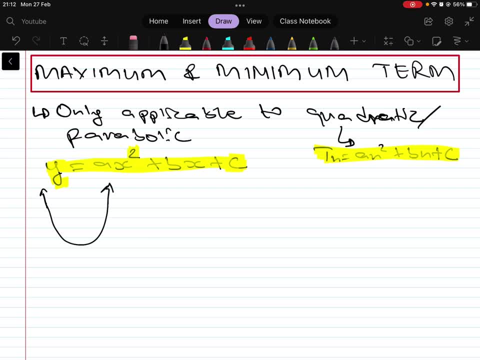 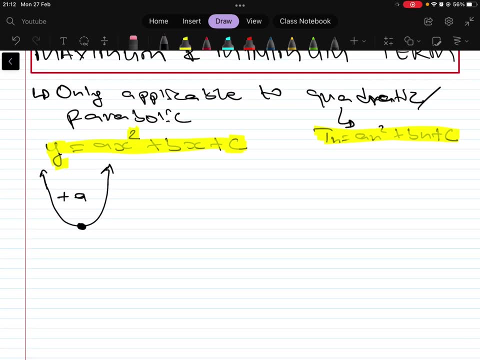 that means the a is positive, that's when it's facing up. and then in that case, that turning point that you have at the bottom there, that is actually your, your, your, minimum point, minimum point. so if it happens that a is negative on the equation the, the graph will look like this: it will face down. 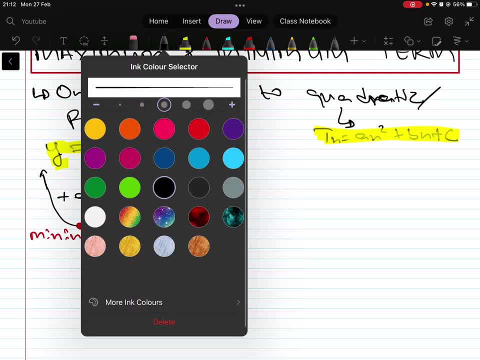 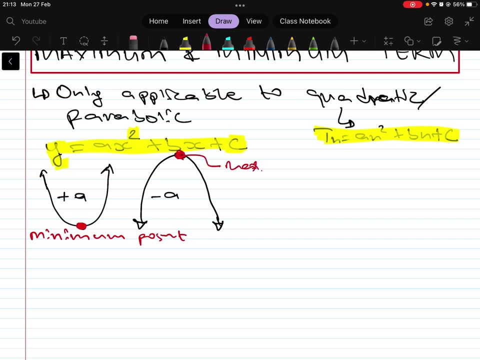 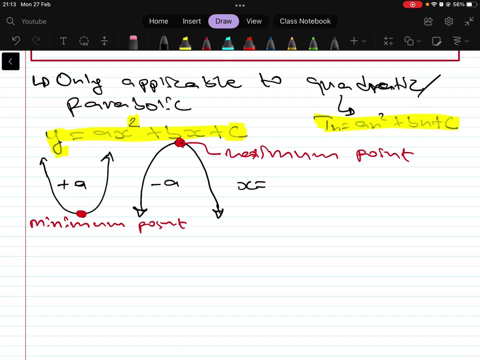 because a is negative, and then you're going to have, um, what you call, rather, a maximum turning point. maximum point, which is the turning point, how you get, uh, the? the turning point is that you remember from functions from grade 10 or grade 11 is that you use the equation minus b. 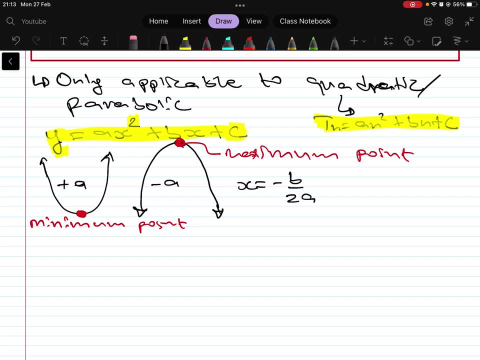 over 2a. that's how you you you get your your turning point. so for quadratic sequences or patterns, we're going to use the same equation. however, instead of n we are using b minus n. i mean n equals to minus b over 2a. that's how you get the position of the turning point. it could either be maximum or minimum. 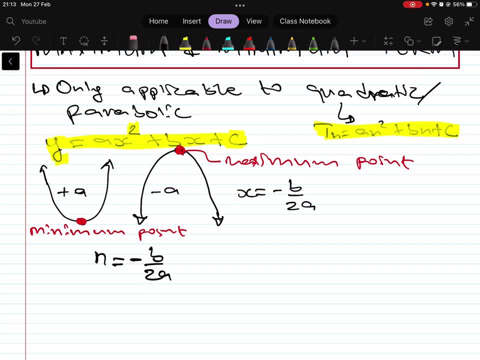 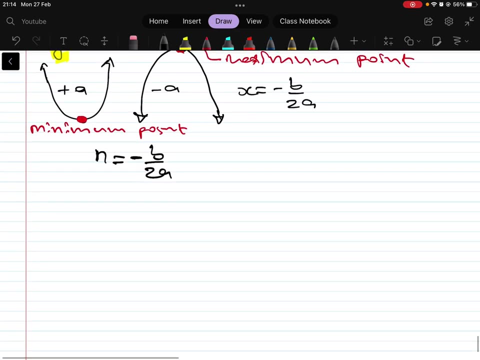 depending on whether or not the a is positive or negative, rather depending on on the, on just a sign of the of the a. so you'll, you'll be given the example, and then you just need to remember that. so let's do the first example. uh, that's our a. let me use rather a instead of one. 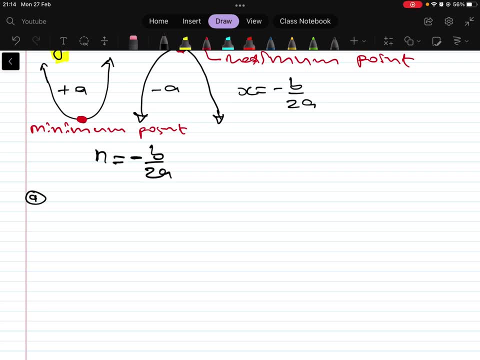 a. that gives us our first example. suppose you are given this. tn equals to n squared minus 10, n minus 30.. um, the questions are as follows, so we're just going to answer them in the odd. which term is the minimum? which term is the minimum term? secondly, 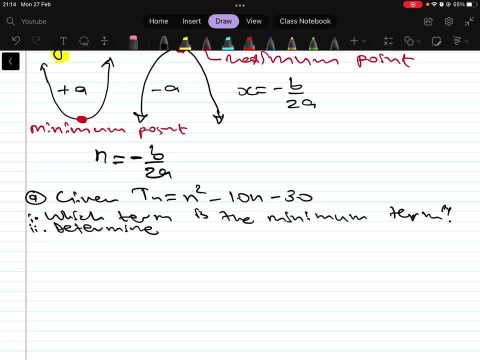 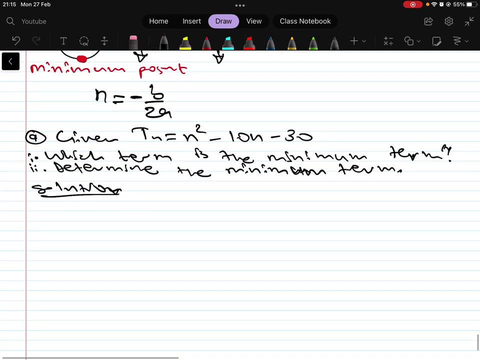 they're asking you to determine. determine the maximum, the minimum term, not the maximum, the minimum, the minimum term. okay, let's try to solve this. they're asking us: um, which term is the minimum to answer the question? basically, what they're asking us here is to get the position. 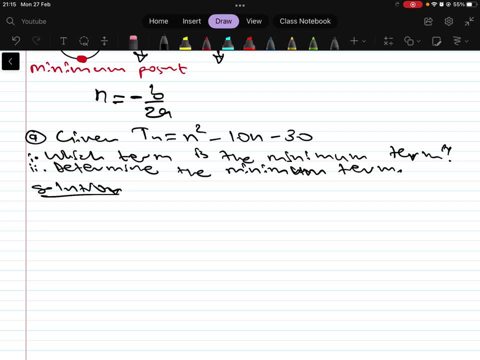 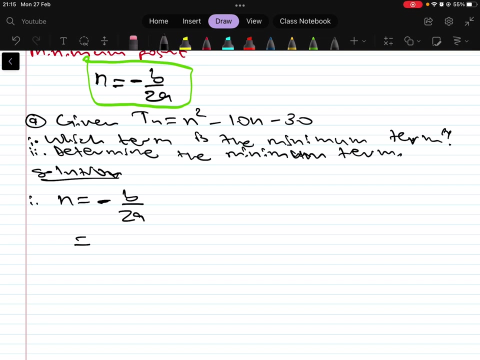 of the minimum term. that is, uh, how, how we get the position of the minimum term. it's as shown by this. so to get the minimum term, we're just going to use the, the equation. that's how we get the position of the minimum term minus b over 2a. we know that in our given equation, our b, it's actually negative 10.. 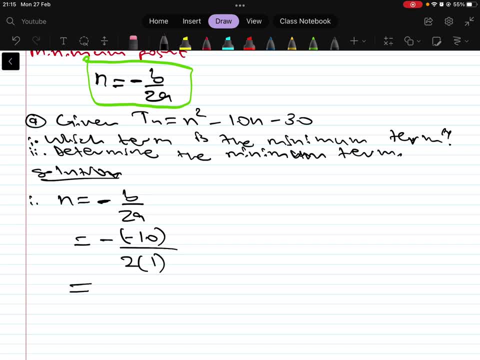 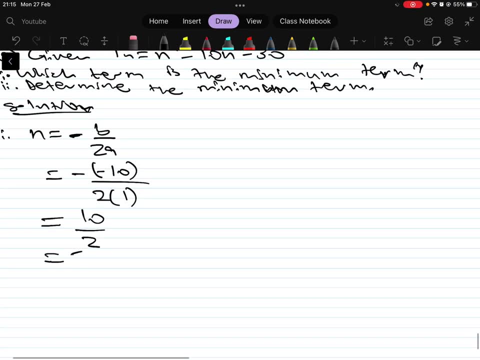 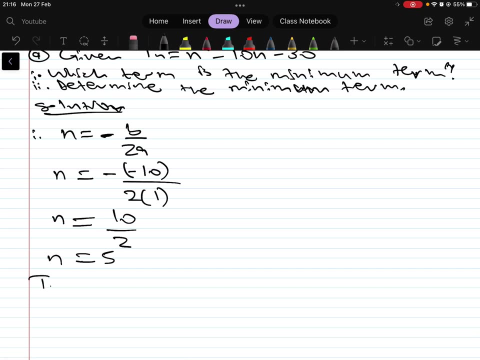 use brackets to get the right answers and our a is just one. so negative 10 times negative 1, just positive 10. then now we have our n being equals to 5.. so that gives us the position of the minimum to answer the question fully. that means term number five. 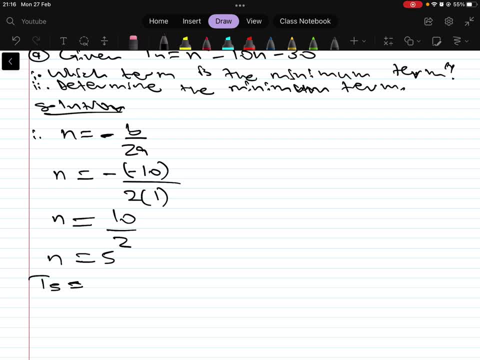 is: uh, term number five equals to the minimum. uh, let me rather write profile: 10 number 5 equals the minimum 10.. so when they ask you which time is the minimum 10, you will tell them that term number five is actually the minimum term you have. you are directing. 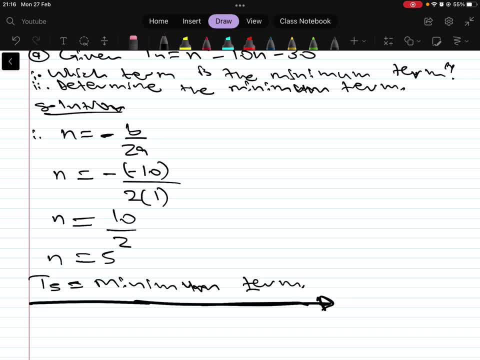 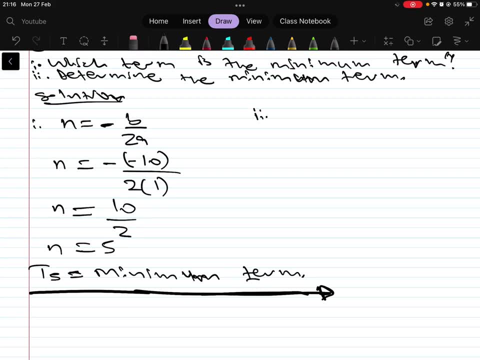 whoever is asking the question to the term which is the minimum term. that means you have answered the question. i hope that's clear enough. and then um, secondly, we are being asked to determine that minimum term. we are being asked: which term is the minimum term? now we're being asked to get. 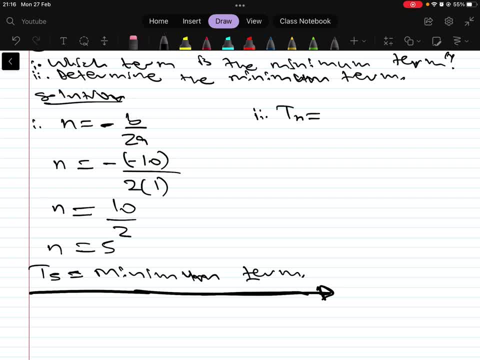 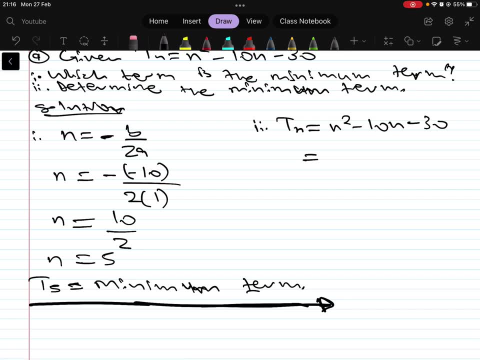 the value of the minimum term. to get the value of the minimum term we are going to use the general formula, which is given as n squared minus 10 and minus 30, because that's what gives us the value of each term. so minimum term is term number five. so the value of that minimum term it's um. 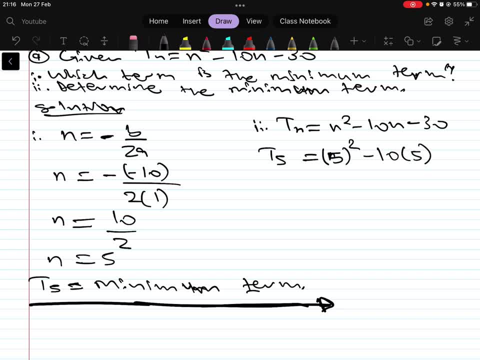 five squared minus 10. we just substitute five in the place of n. then now what is the answer? the answer is actually negative 55. that's our term number five. therefore, to respond, we say: a minimum term equals to negative 55. you, but mathematically, even if you were to leave it here, it should still be fine, because we're not. 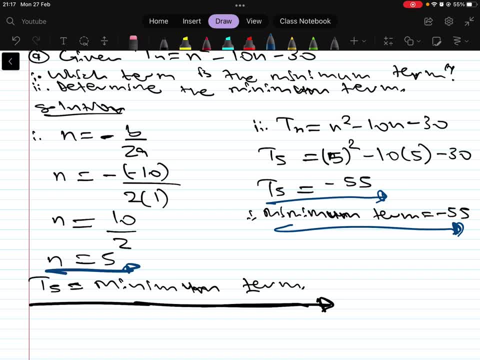 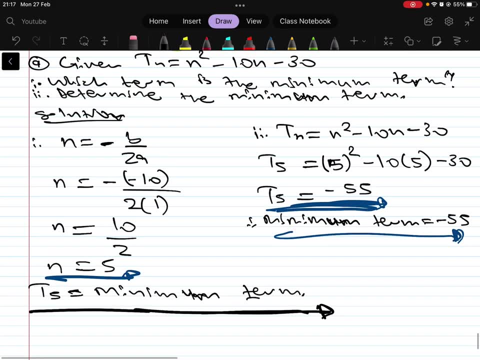 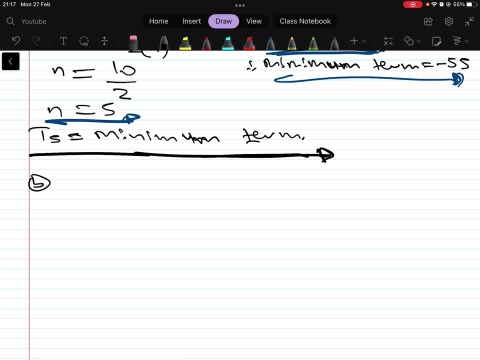 really trying to do english so you could leave the answers exactly there and then you should still be fine. but writing it like that shows that you actually understand what you were calculating. you're not just doing the calculations. let's move on to another example. um b, you are given tn. 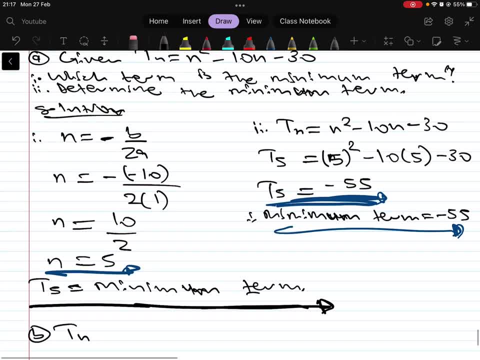 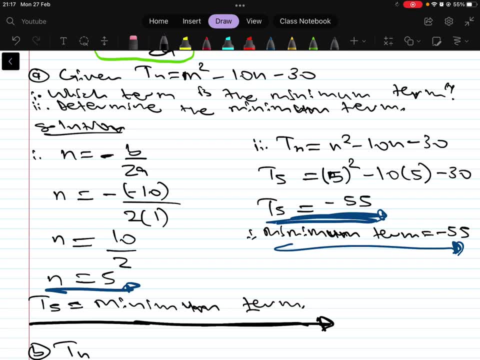 uh, before we move on, actually i just wanted to state something: the they asked you to determine the minimum term because the a is actually positive here. it's positive one. that's why you are being asked to calculate the minimum term. if it's positive, remember, if it's positive. 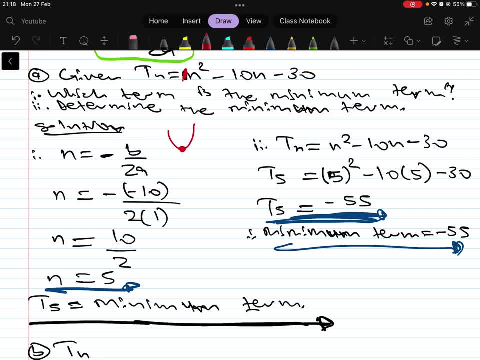 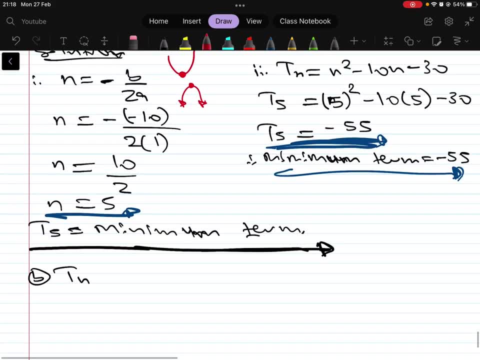 it's facing合, then that term is the minimum. if your a was negative, you'll have it like that. then this term becomes your maximum, like that. so, depending on the value of a, they will either ask you to get the minimum or the maximum. okay, let's continue to that. another example: um. i wanted to write it in four times. 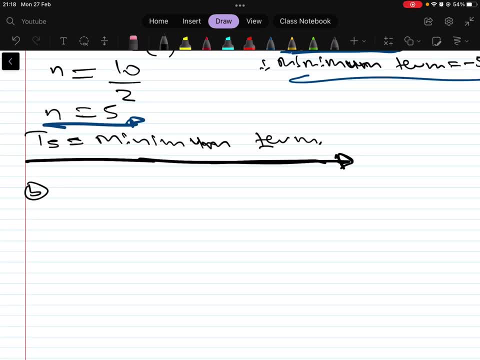 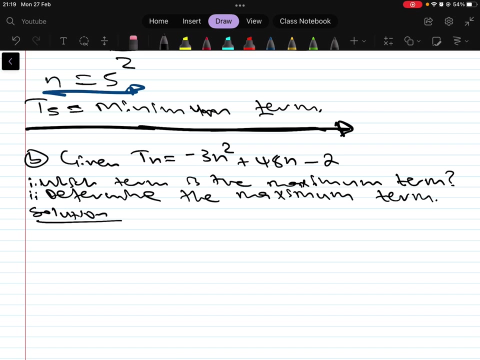 my. i wanted to write it in four times. given T, n equals to negative, 3 n squared plus 48, n minus 2, they still ask similar questions: which 10 is the maximum? 10 determine the maximum 10. okay, so for the same explanation, or from the same explanation. 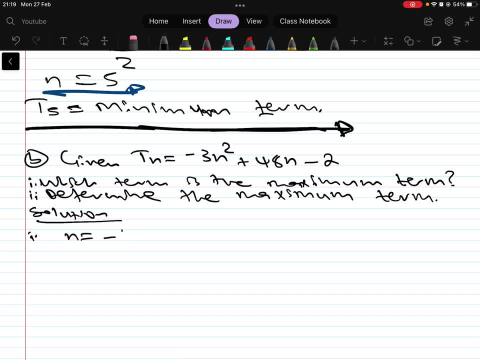 okay, so, from the same explanation, or from the same explanation, or from the same explanation, or from the same explanation that we know that, to get the explanation that we know that, to get the explanation that we know that, to get the position of the maximum 10, this: 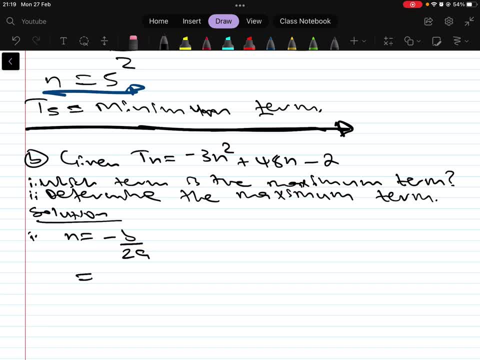 position of the maximum 10, this position of the maximum 10, this equation works, whether you are getting equation works, whether you are getting equation works, whether you are getting the position of the maximum time of the, the position of the maximum time of the, the position of the maximum time of the minimum 10, because the whole point is to 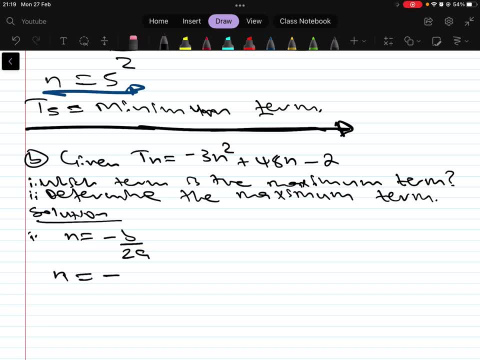 minimum 10, because the whole point is to minimum 10. because the whole point is to get the position of the turning point. so get the position of the turning point. so get the position of the turning point. so the turning point is either maximum or the turning point is either maximum or 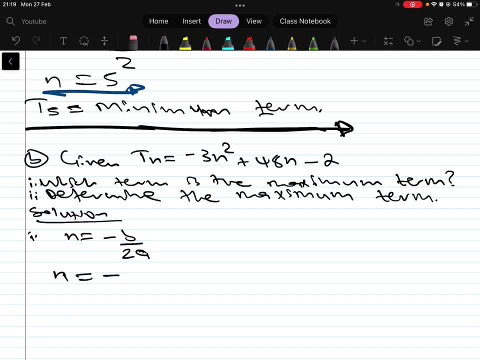 the turning point is either maximum or minimum. it's maximum or minimum minimum. it's maximum or minimum minimum. it's maximum or minimum, depending on the value of a, if it's positive or negative. so in this question our b is 48, our a is negative, 3. that's why, because it's 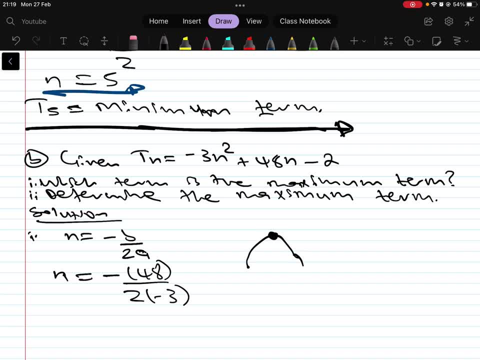 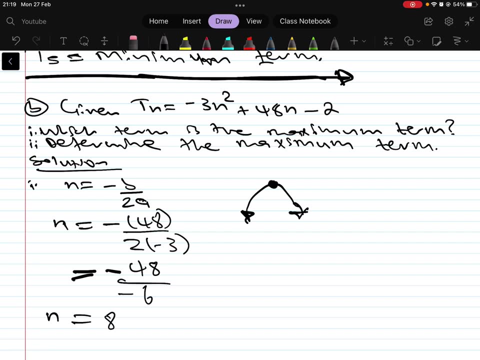 negative. it's facing: uh, down that point. it's going to be our maximum point. so negative 48, we're going to have something like that: negative 6. and then now what would be our answer? our answer is 8. that means our n is 8, so term number 8: it's actually the, the maximum. 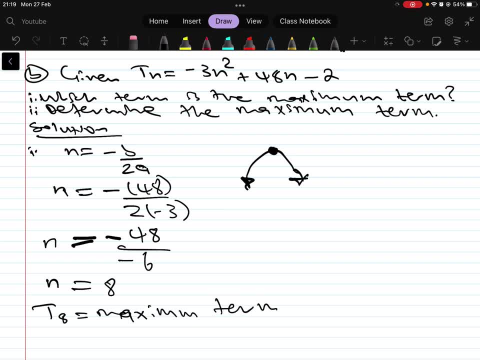 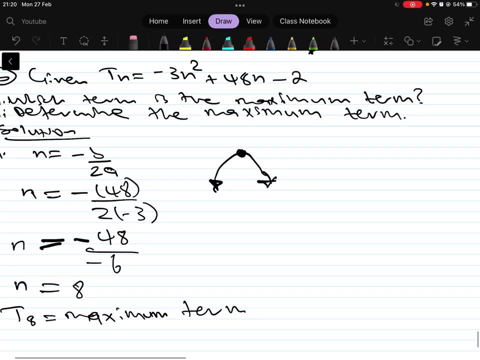 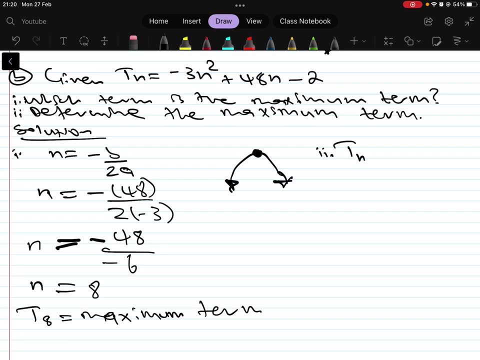 term maximum. just get the spelling right. i keep just writing things because i'm in a hard try to not make the video too long, okay, and then uh, now being asked to get the the term or the maximum term, we're just gonna use the equation like we did previously. 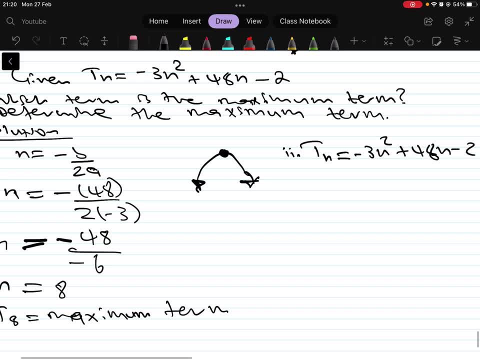 that's 48 n minus 48, n minus 2, so we have minus 3, which is term number 8. that means we have 8 squared plus 48. times 8 minus 2, the answer is 190, that's term number 8. therefore, um, okay. 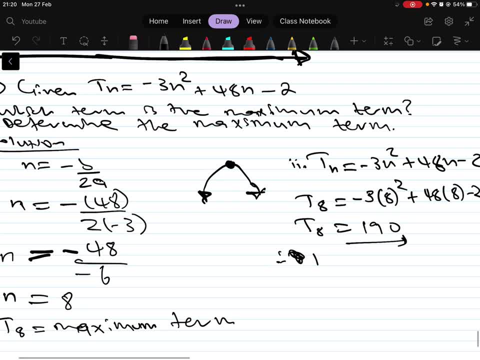 therefore, what do we say? 190 is the maximum term, but you don't need to write this. this is the maximum term, but you don't need to write this. this is the maximum term, but you don't need to write this. you can just stop here. so let's move on and stop doing unnecessary things. 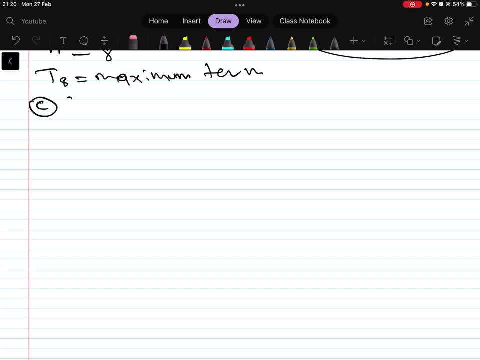 okay, um suppose you're given this. that's another example. tn equals to 5n squared minus 50, n plus 1, right. and then here you're only being asked this question: does the sequence have a, have a maximum or minimum term? and y? so it has what it has, because we look at the a. 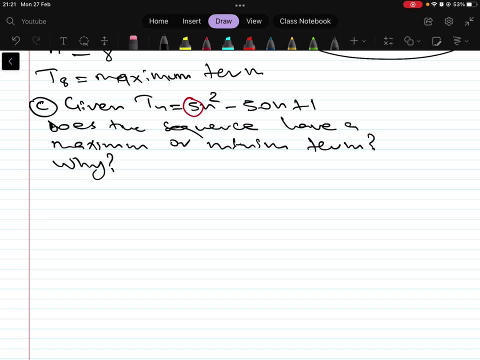 so it has what it has because we look at the a, so it has what it has. because we look at the a to see if it's positive or negative, then we can to see if it's positive or negative, then we can. to see if it's positive or negative, then we can conclude the a is positive. if it's positive, it conclude: the a is positive. if it's positive, it conclude the a is positive. if it's positive, it means the whole, means the whole means the whole graph. if we were to plot it, it's going to graph. if we were to plot it, it's going to. 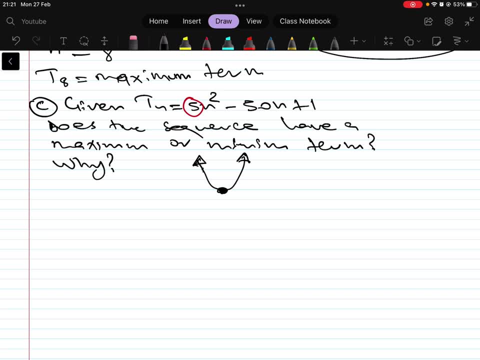 graph. if we were to plot it it's going to face up. then we have what the minimum face up, then we have what the minimum face up, then we have what the minimum term there. so it has a minimum minimum, minimum 10. reason: the a is greater than 0. it's positive to a. see I.